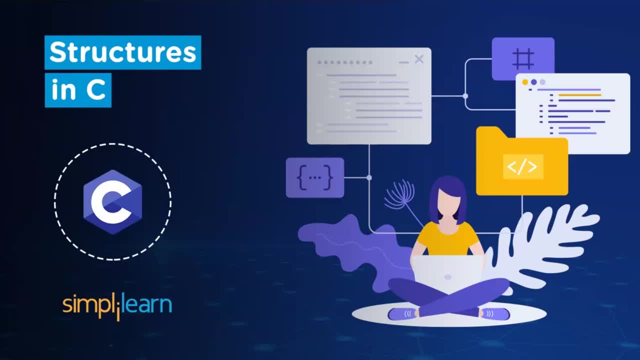 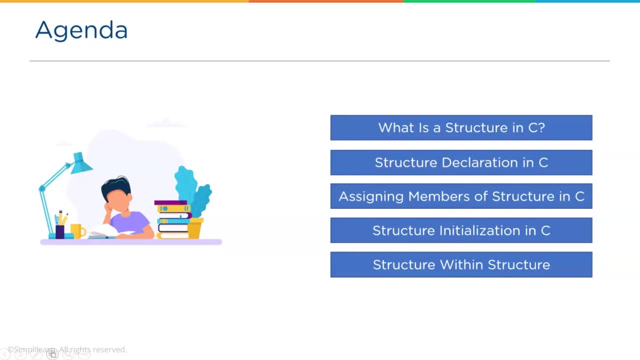 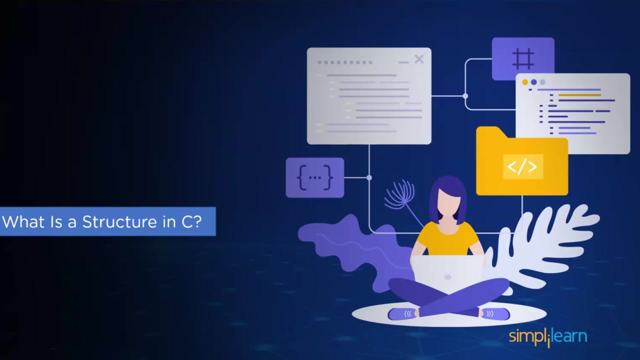 miss an update. So now, without any further delay, let's begin. This session will help you to understand what a structure is in C. Then let's understand the general syntax of structure declaration, After that assigning members of the structure in C, Later structure initialization and finally, structure within structure. 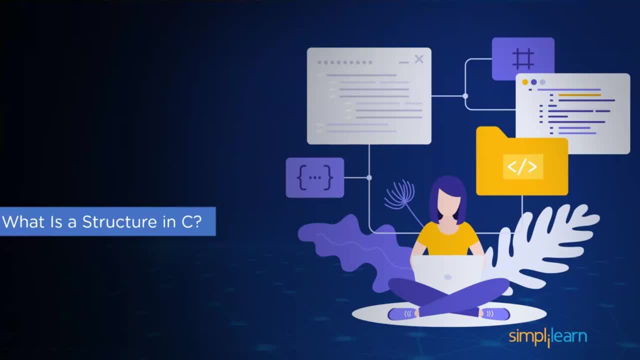 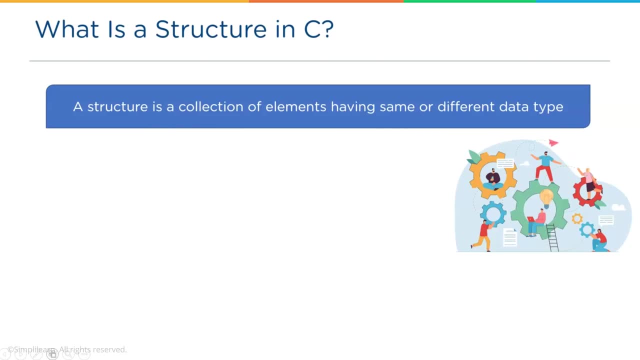 Now let's begin by understanding what a structure is. in C, As we all know, array is a collection of elements of the same data type. Similarly, a structure is a collection of elements of the same or different data types. For example, unlike an array, a structure can have members. 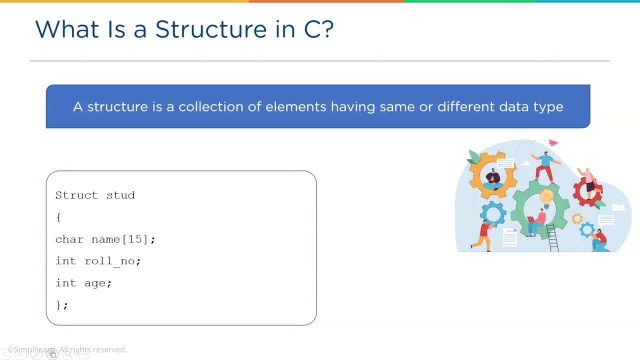 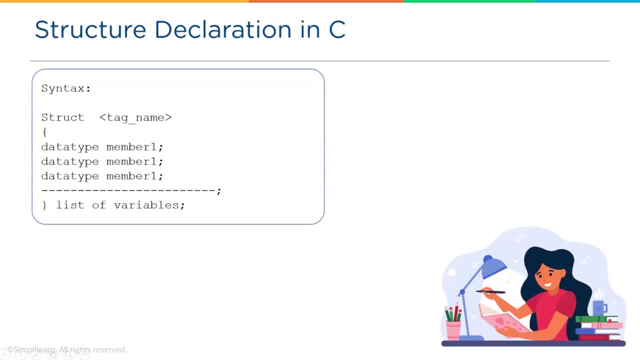 of different data types like int, float, char, etc. Now let's have a look at structure declaration. in C We use the struct keyword before the tag name to define a structure. Tag name is nothing but a structure name. Whatever is declared inside the struct, curly brackets are members. 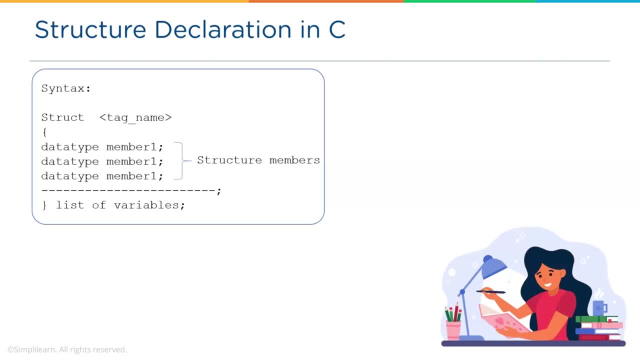 of the structure. Once the members are declared, the weight table has to be created to access the members of the structure. Now let's see the example. We have struct keyword, followed by student as a tag name, then a list of structure members, And they are: name of type, char, role, number and age. 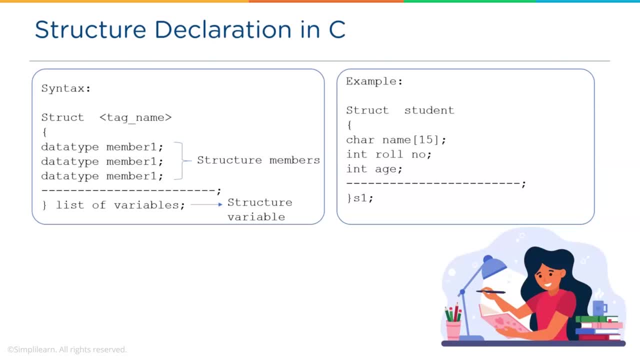 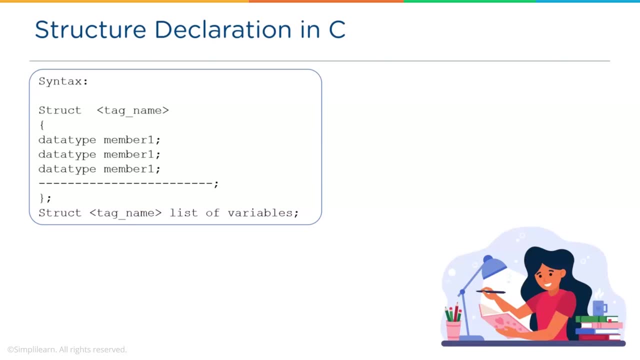 of type int and s1 as a structure variable. We can have a list of structure variables. Another way of structure declaration is we can declare structure variable outside the curly brackets By using struct keyword followed by a tag name, then declare variable list, For example struct keyword, then student tag name and s1. 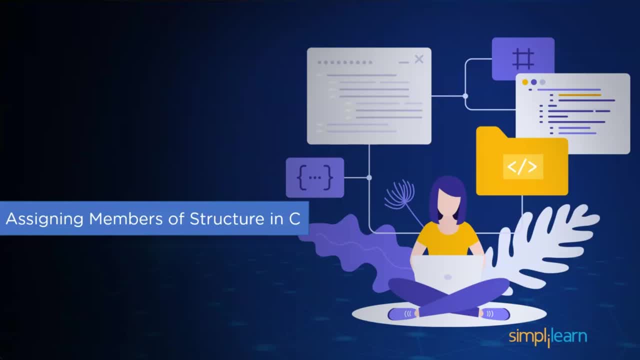 as a variable name In structures. in C programming we cannot assign values during the definition of a structure. It indicates the wrong way to the declaration. So now let us try to understand the right way of assigning values to the structure members in C. 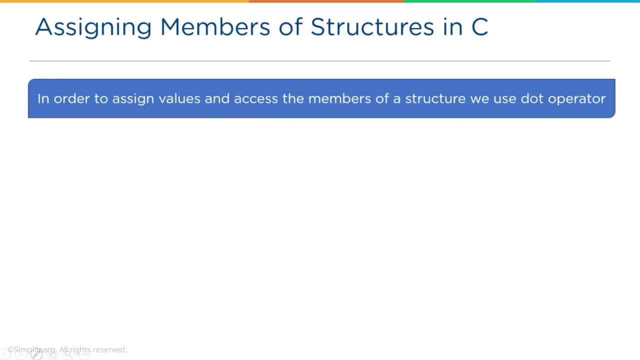 To assign values to all the members of a structure and access, we use dot operator, also known as a period operator. Look at the syntax below to clearly understand how we access and assign the structure members. First the structure variables, followed by the dot operator and structure members. For example, s1 dot role number is equal to 34,. 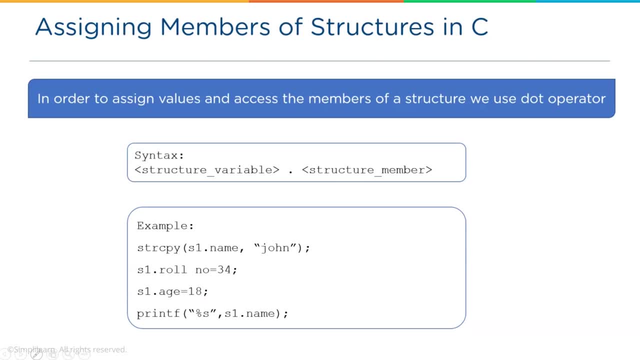 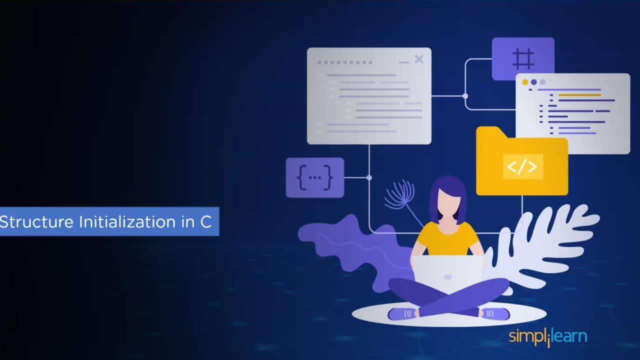 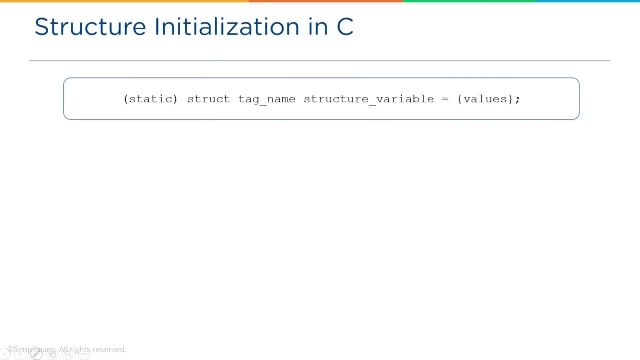 s1 dot age is equal to 18, and we make use of the string function strcpy to copy the name. Next, we have structure initialization. in C We can also initialize the structure variable And to initialize we can directly assign values of all the structure members inside the curly brackets with an assignment operator. 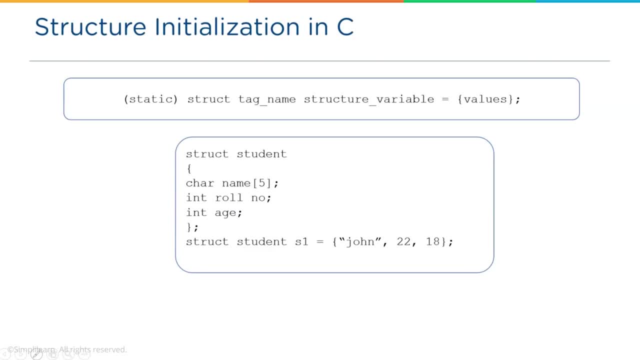 For example, struct, student s1 is equal to. inside the curly brackets, enter the values separated by comma operator. In this particular example, name is John, the role number is 22 and the age is 18.. Now that we know how to declare and initialize. 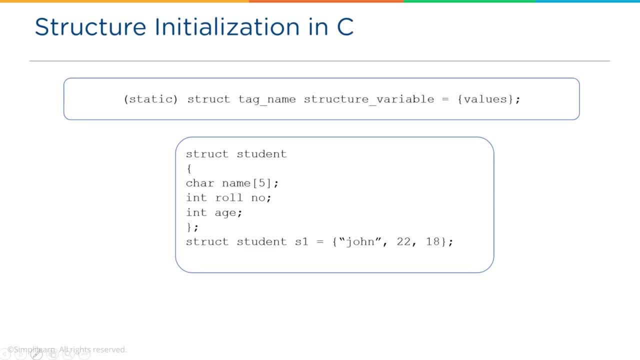 structure variables in C. Let's see how to declare and initialize structure variables in C. We need to trigger this ToễčićII. So this is a surface structure variable, real big C into the wo bas, alright, And the Momoder can turn into example. 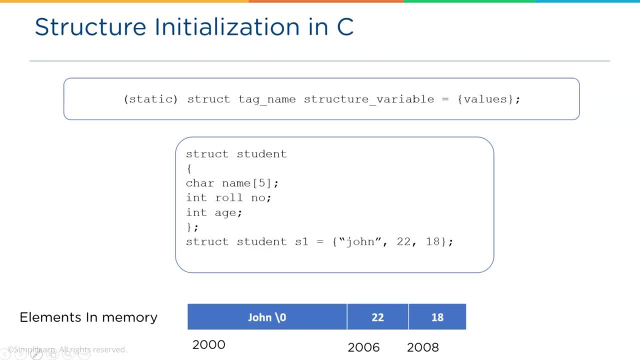 And in the case of the superb, except the s1 variable, the amy gets uneaval. So once again I'll show you how it works by taking the structure primeira somewhere outside the matrix. Today, C will have some elements in this case, or at least we will get some memory elements. 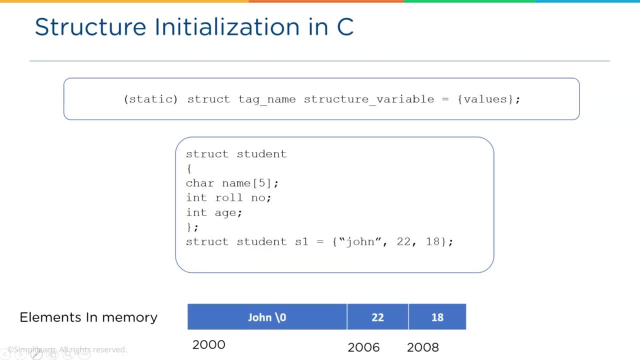 So N takes one byte of memory space according to size of the string the characters will occupy in the memory. In structures the memory is created once this structure variable is, ie 5 bytes for s1.nick, 2 bytes for s1.rollNumber and 2 bytes for s1.h. 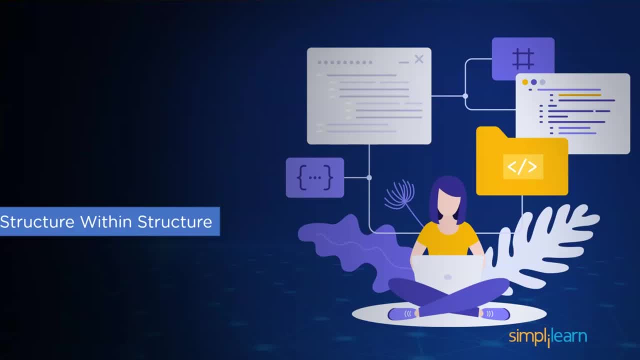 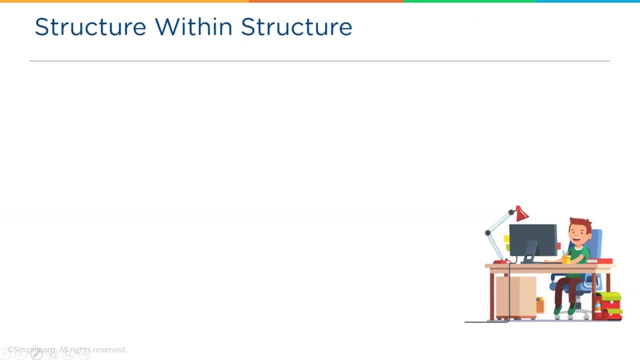 So I think you got a good understanding of how memory is allocated for the structure elements. Okay, so let us move on to the structure within structure. in C, When a structure contains another structure as a member, it is known as a nested structure or structure within a structure. 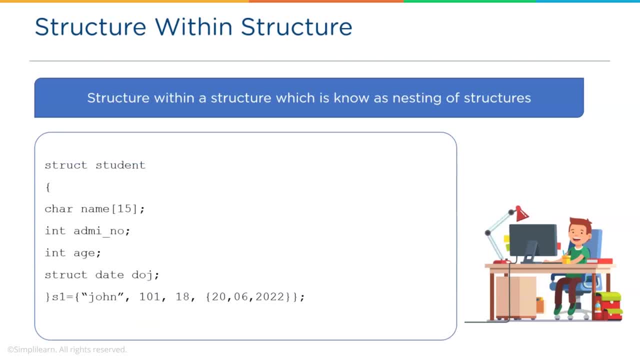 For example, let's consider a structure named student and another structure named as a date. In this example, a structured date acts as a member, So a structured date has its own members and they are date, month and year of typing And structure variable for date is doj. 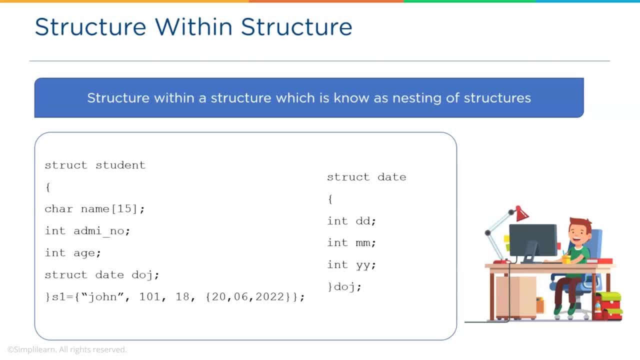 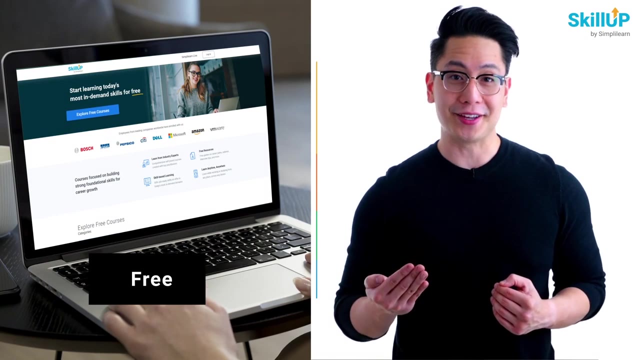 And this structure variable is initialized for both the members of the structure, That is, name, admission number, age, date, month and year. Now let's execute a simple structure program. If getting your learning started is half the battle, what if you could do that for free?